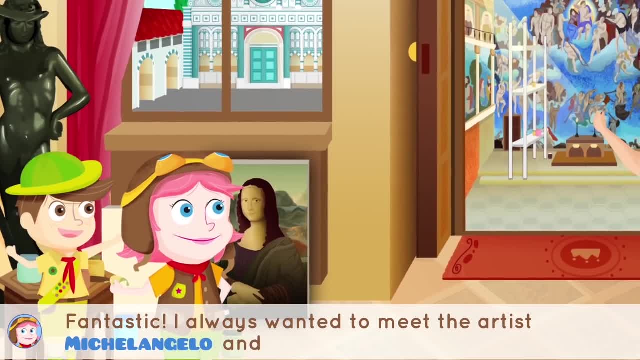 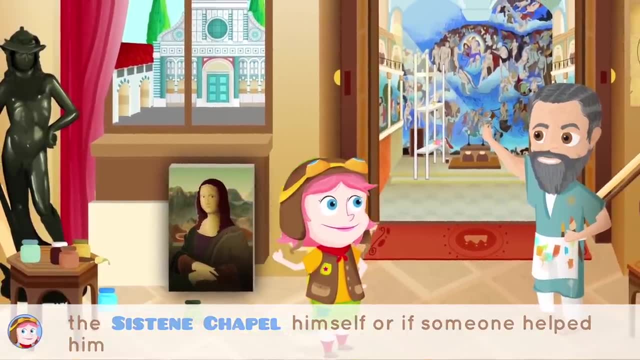 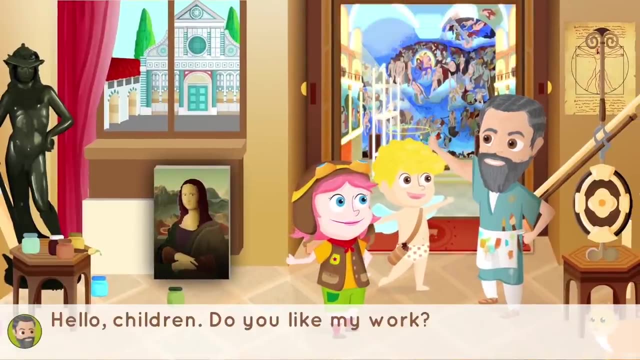 Fantastic. I always wanted to meet the artist Michelangelo and ask him if he painted the Sistine Chapel himself or if someone helped him. Hello children, Do you like my work? I did it all myself, even though it took four years. 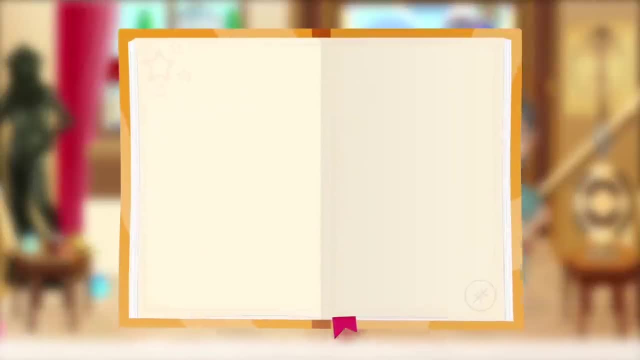 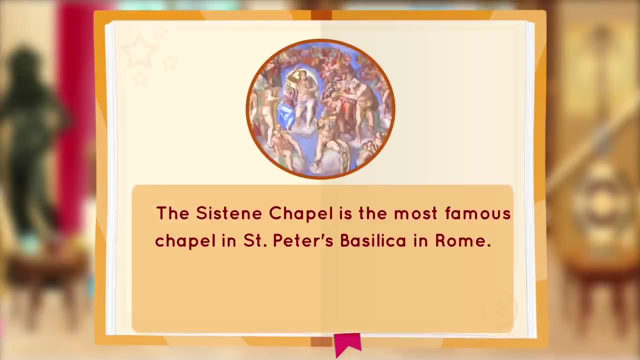 Hello children, Do you like my work? I did it all myself, even though it took four years. The Sistine Chapel is the most famous chapel in St Peter's Basilica in Rome. Its ceiling is a series of fresco paintings by Michelangelo. 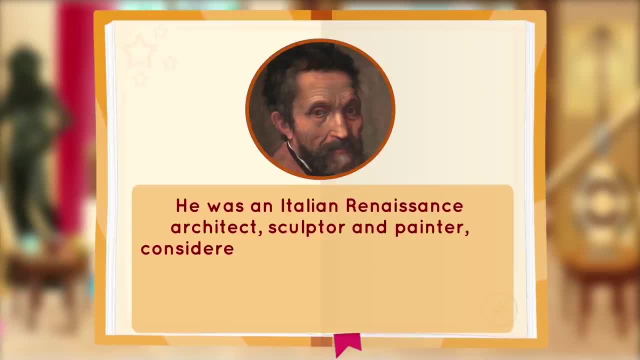 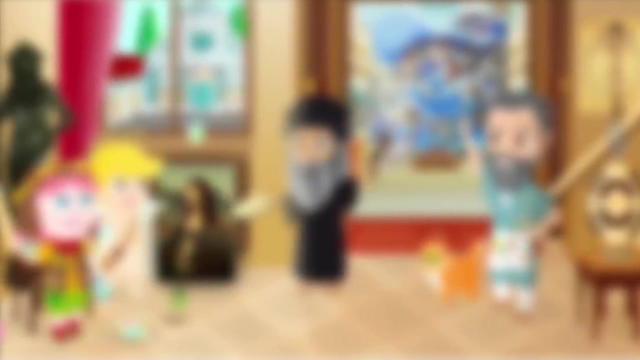 He was an Italian Renaissance architect, sculptor and painter, considered one of the greatest artists of all time. His most famous sculpture is David and his most famous painting, The Ones in the Sistine Chapel. His most famous sculpture is David and his most famous painting, The Ones in the Sistine Chapel. 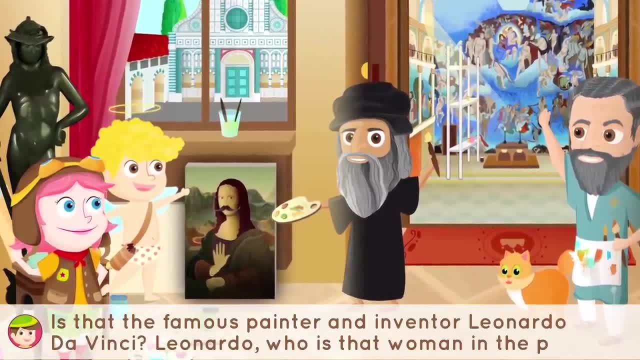 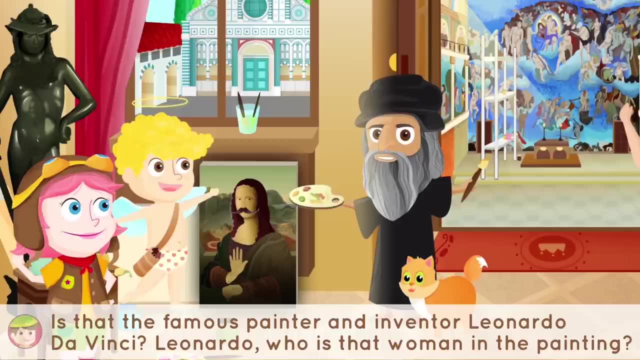 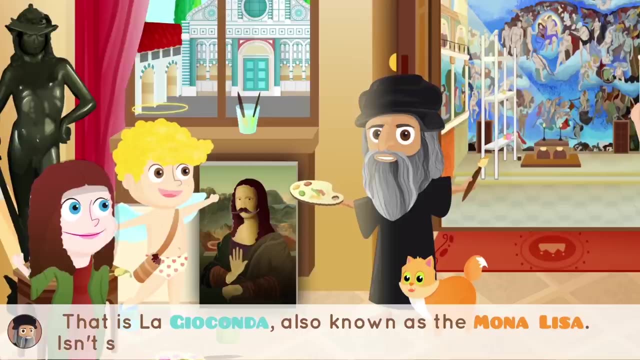 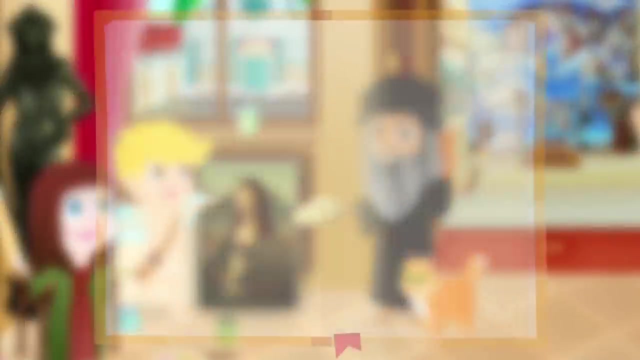 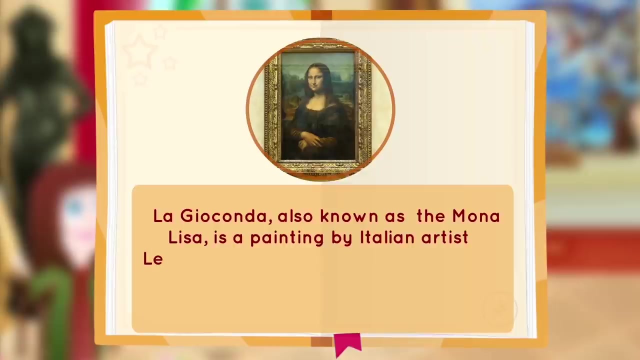 Is that the famous painter and inventor Leonardo da Vinci? Leonardo, who is that woman in the painting? That is La Gioconda, also known as La Mona Lisa. Isn't she beautiful? La Gioconda, also known as The Mona Lisa, is a painting by Italian artist Leonardo da Vinci. 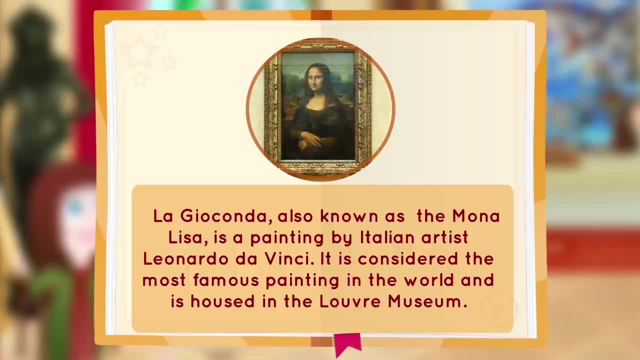 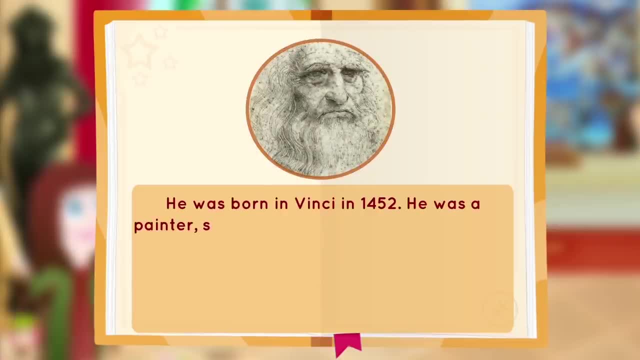 It is considered the most famous painting in the world and is housed in the Louvre Museum. He was born in Vinci in 1452.. He was a painter, sculptor, inventor, architect, musician, anatomist, chef, philosopher, which is why he is known as a Renaissance man. 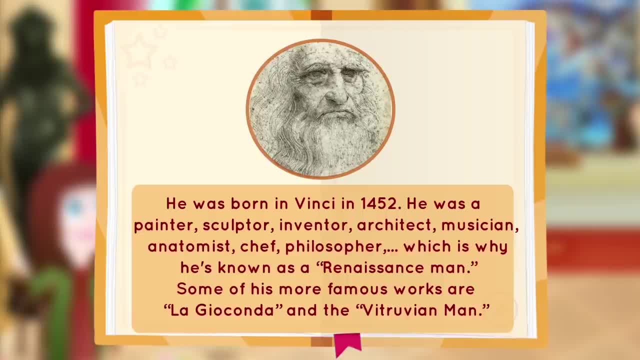 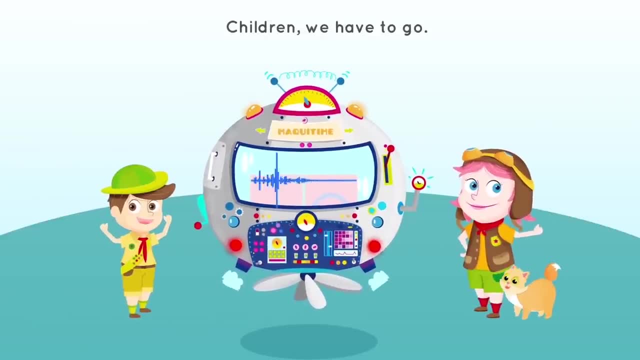 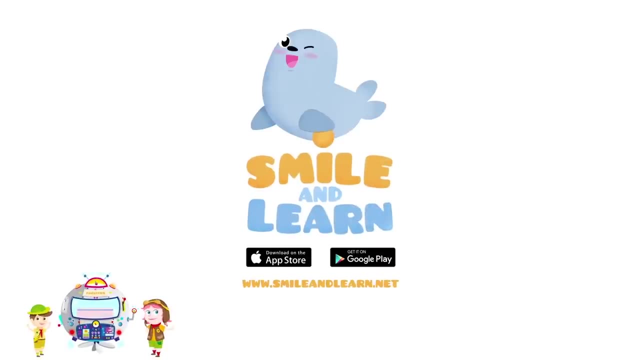 Some of his more famous works are La Gioconda and The Vitruvian Man. Children, we have to go Well, children. are you ready to discover more periods from the past? Click on the box to keep traveling through time. Subscribe to our channel for more videos like this.